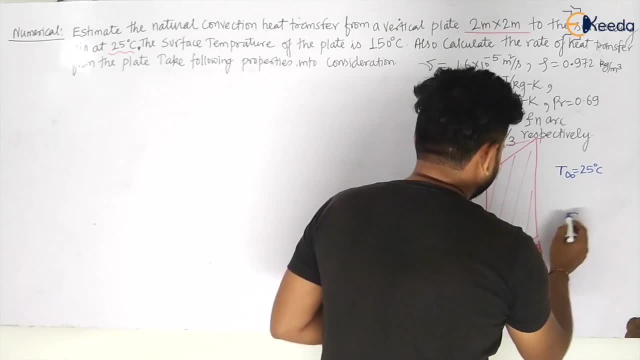 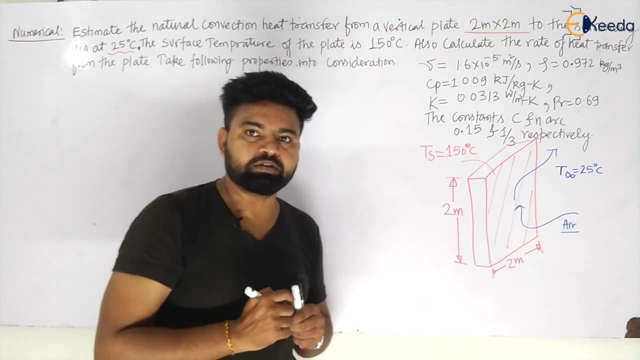 transfer so let us see this transfer like air will come with � represent the rate of q darker for forty degrees or higher per second so like this there will be cooling of the plate there will be cooling of the plate let us see my dear students so there will be cooling and so let us see what 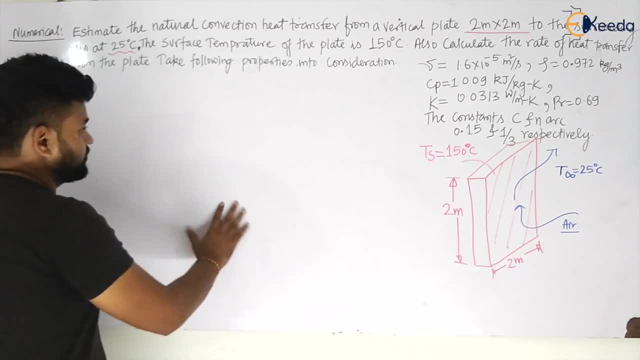 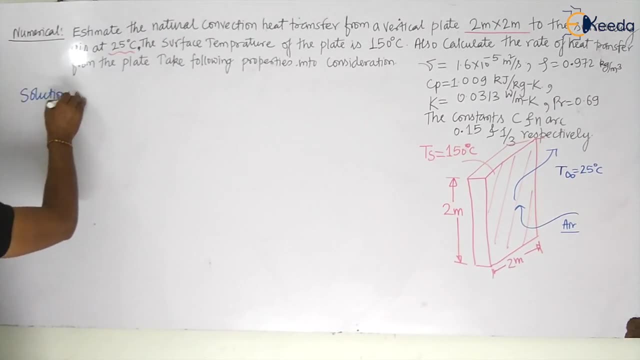 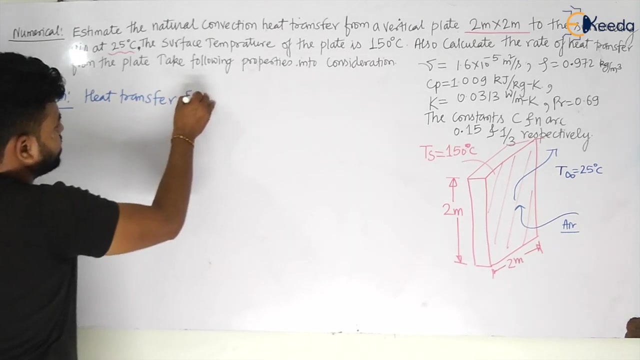 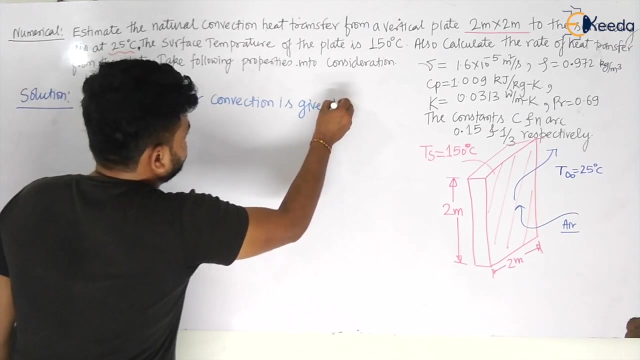 will happen here. we have given these properties. we have to calculate the heat transfer. so let us see how heat transfer is given by my dear students. so the heat transfer is even by Turkey. convection, for convection is given by, is given by. that is Newton's law of cooling. 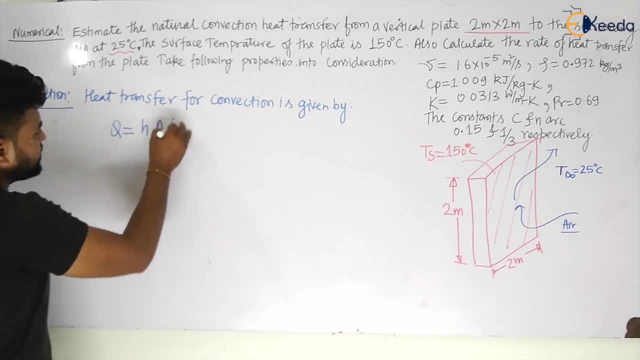 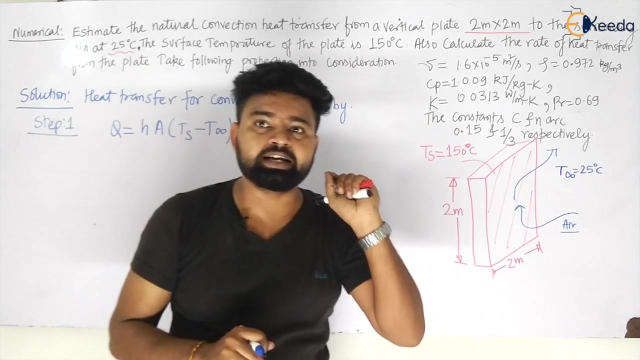 that is given by HA into TS minus T infinite, minus TS minus T infinite. so that was your, let us say, step one for natural convection now. but you don't know the value of H, that is heat transfer coefficient. he has not given my dear students heat transfer coefficient. he has not given this will be equal to: 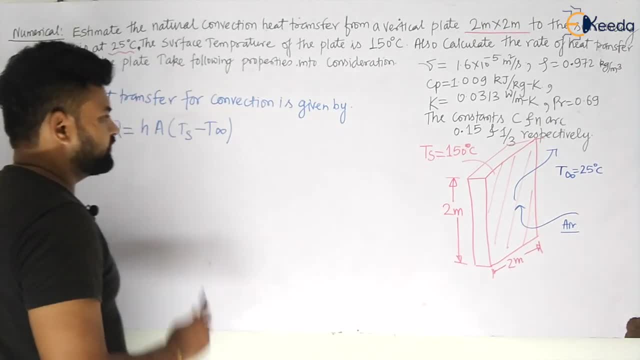 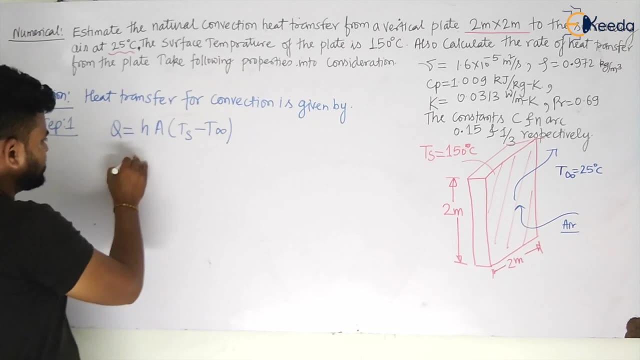 what? let us see. so heat transfer coefficient he has not given. now what will happen when heat transfer coefficient he has not given? you have to calculate it, and we know that Nusselt number is nothing but equal to heat transfer coefficient multiplied by characteristic length. my dear students, LC divided by K of fluid. 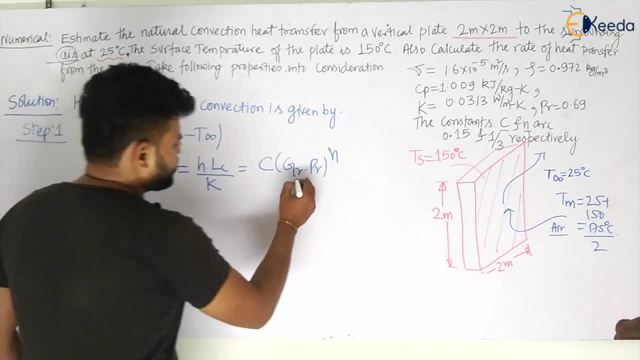 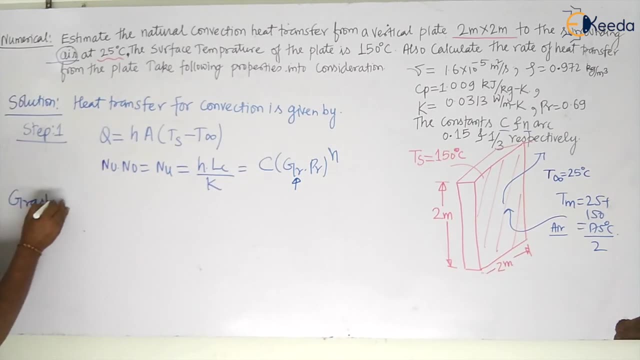 conductivity of fluid. so we have to calculate G R, my dear students, that is your Grashof number and what is your Grashof number is given by. so the Grashof number is given by, Grashof number is given by. is given by my dear students, that is, G R is equal to G beta TS minus T, infinite LC to the. 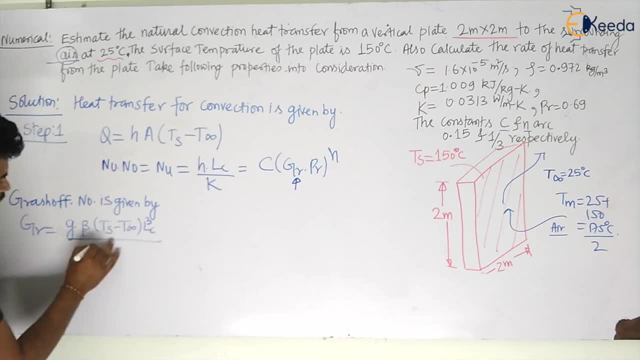 power 3, divided by nu square, my dear students, divided by nu square. so what is the value of beta, my dear students? so what they have given? so they have given provin here. There they have your idea of spreads, and we know. then air can be treated as. 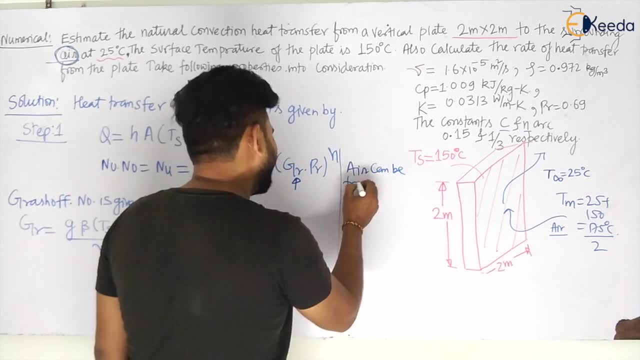 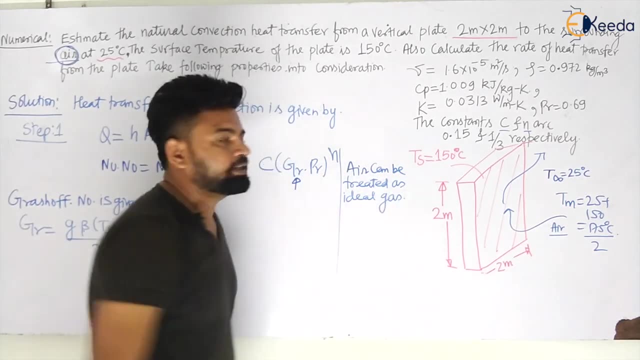 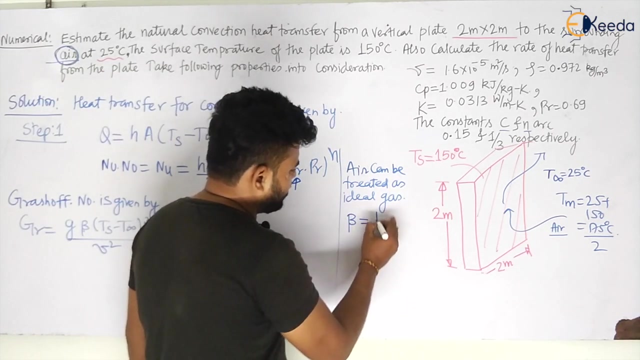 was here, can be treated as I deal. yes, my dear experience, and where the cavities as I do. this Navik alab Omega coefficient of volume, explicitly, that is, your beta, and beta is given by 1 upon P, where P is the mean temperature, my dear. 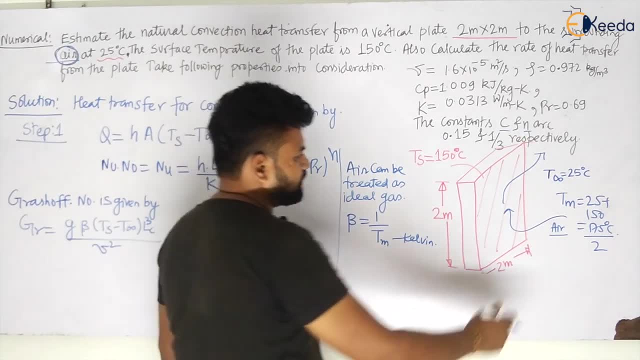 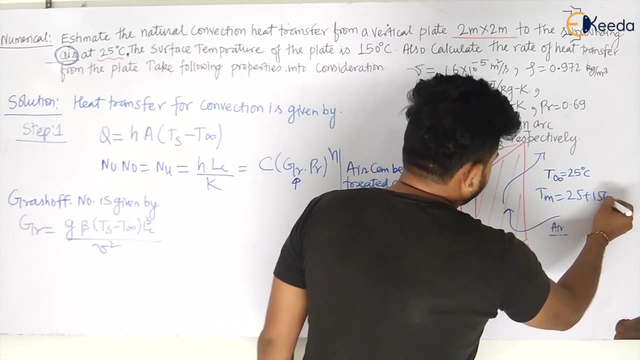 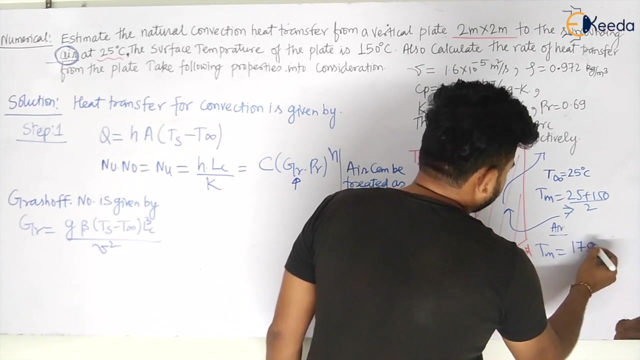 in Kelvin. T is the mean temperature in Kelvin And what is the mean temperature in Kelvin? So you can easily calculate here. So mean temperature will be given by 25 plus 150. that is divided by 2.. So Tm will become equal to 175 divided by 2, my dear students. So 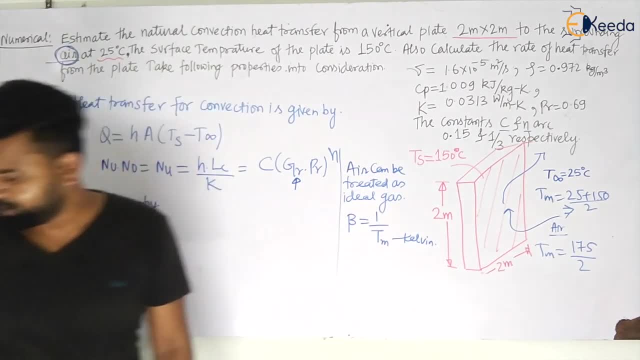 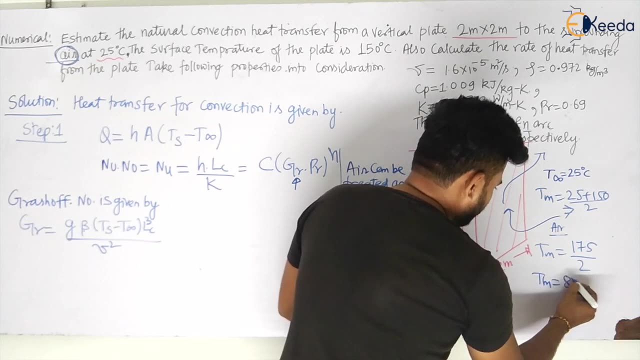 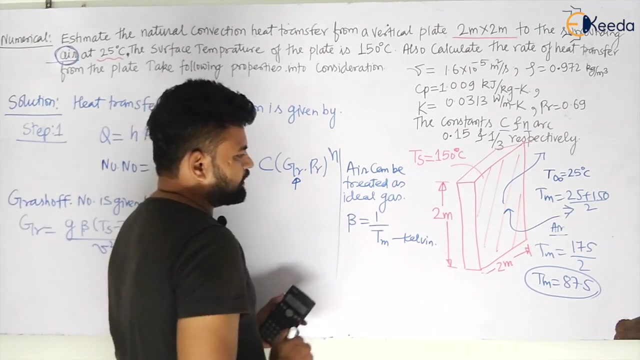 this will be how much. Let us calculate it. So Tm will be equal to 175 divided by 2. This will be equal to 87.5, my dear students, because all the properties will be calculated at the mean temperature. So this is in degree Celsius, my dear students, Let us put, take. 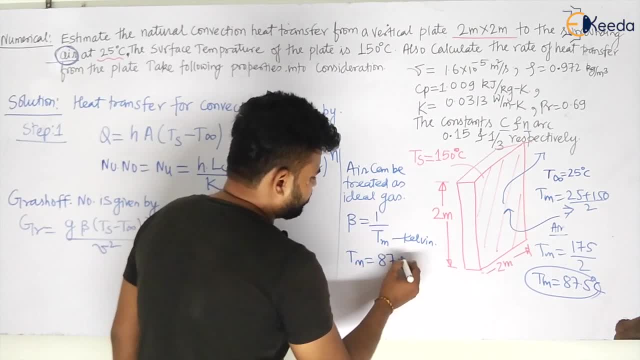 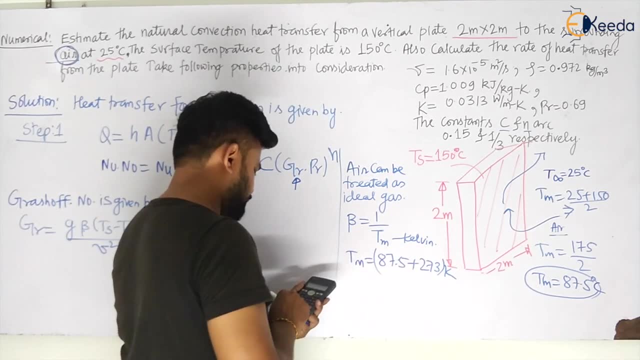 it in Kelvin. So Tm will become equal to 87.5 plus 0.5 plus 273, and this value will be in Kelvin there, plus 273, and this value will be in Kelvin. This will be 360.5. my dear. 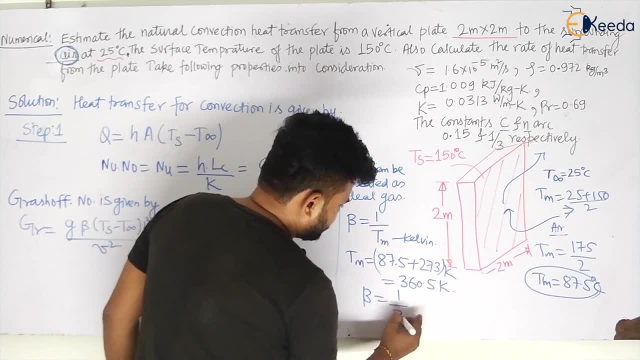 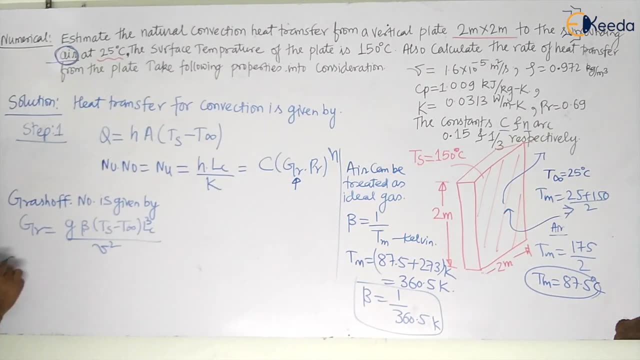 students, Kelvin. So beta will be equal to nothing but 1 by 360.5, Kelvin, my dear students. So let us put this value here in gash of number and let us put all the values in calculator gash of number. So gash of number will be given by 9.81 into beta, which is 1 divided by 360.5. 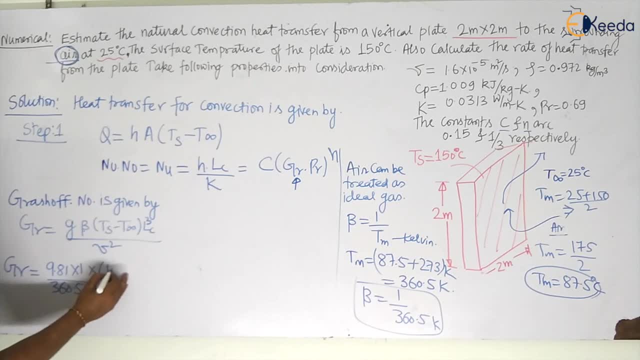 Kelvin into Ts minus T infinite. What is Ts 150 minus 25 multiplied by LC cube? that is 2 cube, my dear students, 2 cube, 2 cube divided by mu square. What is the value of mu 1.6 into Tm minus 5, whole square? So 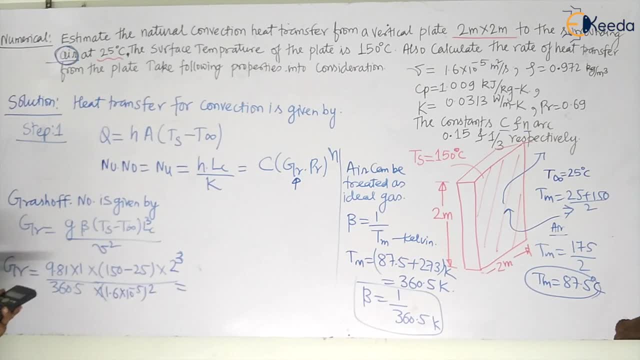 you will have your gash of number from here and let us calculate it. So this will be 1.6 into Tm minus 5 whole square. Okay, and this will be 9.81 into 1 into 9.81 into this. 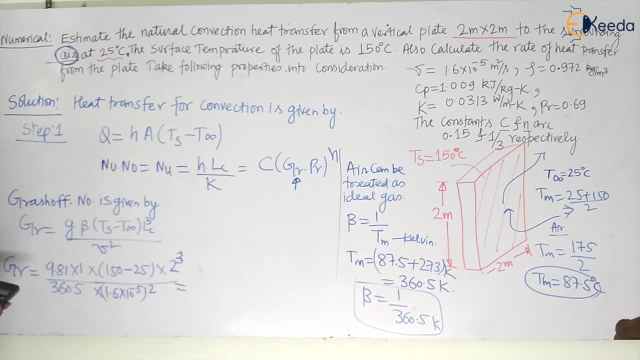 will become 125 into this will become 8, my dear students. So this will be 1.6 into Tm minus 5 whole square. Okay, Now we are going to get our gash of number. Are you understanding everything? 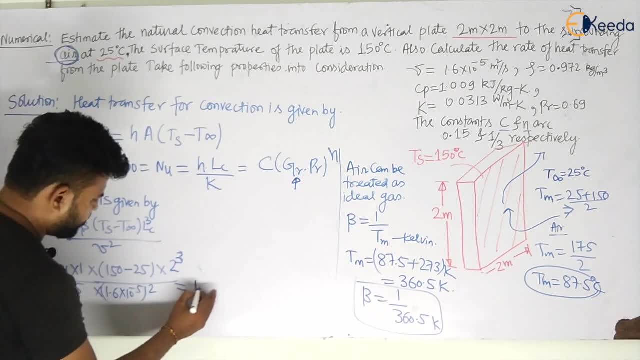 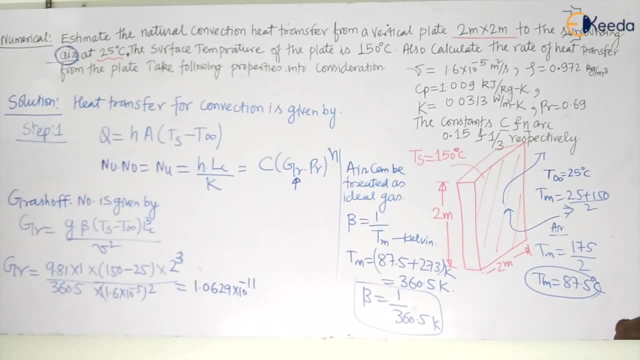 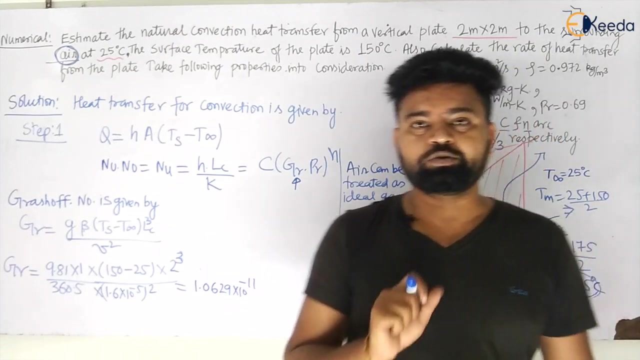 We are going to write camouflagingatchedn. for this first, let us spend one time, Okay. and for this first we are going to get our greash of number. So what we need to do is we are going to put this in our calculator. So para 1 plus 3 times capital, A plus c. 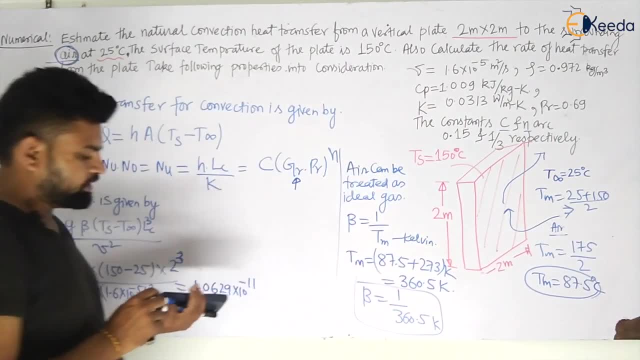 minus n minus 4 divided by L is equal to then minus i, multiplied by 2, by 24 times Armali power. So in this particular case, this is first time. So what we have to do is by multiplying this out. We will spell it with gash of number: send x plus t, minus i plus l over 1 times 3 is. 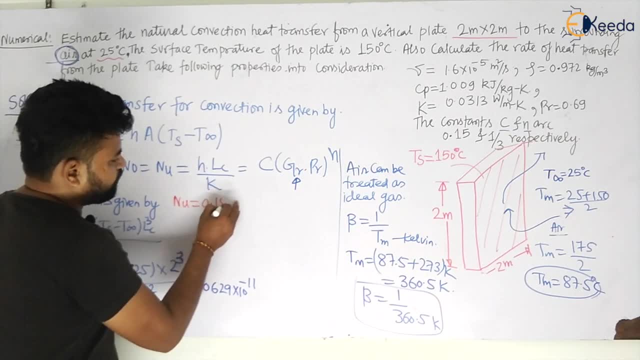 equal to never. we just have nothing but 1 plus people, 7 times 9.. We are sending these. Gash will be given by C, which is given to be 0.15,, my dear students, and N is given to be 1 by. 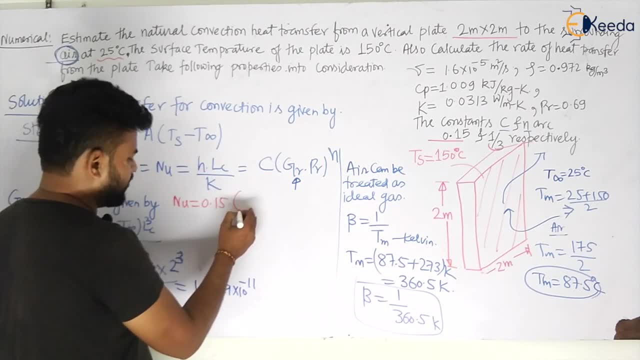 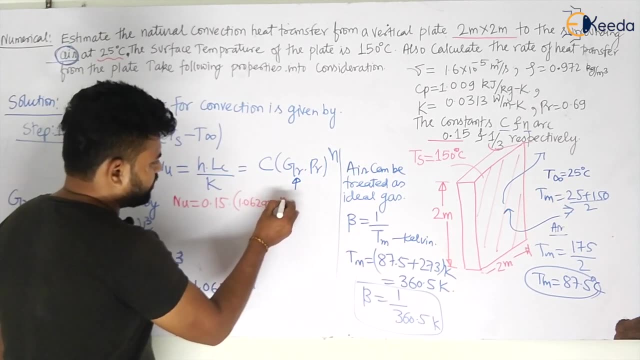 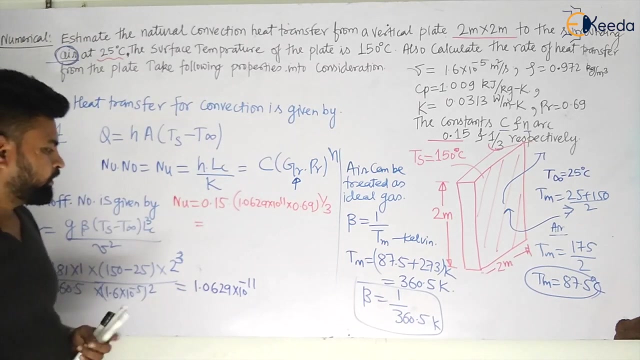 3. So C into G car, which is 1.0269, 1.0629, into 10 to the power 11, multiply PR 0.69 to the power 1 by 3,. my dear students, Let us see what will be the value of this into. 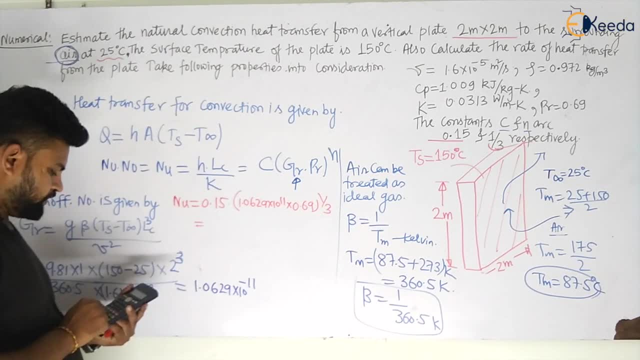 0.69, 0.69, to the power 1 by 3, 1 by 3, 1 by 3,, my dear students, and that is plus 11, that is not minus 11.. So this will become 4185, multiply by C 0.15.. So you will have. 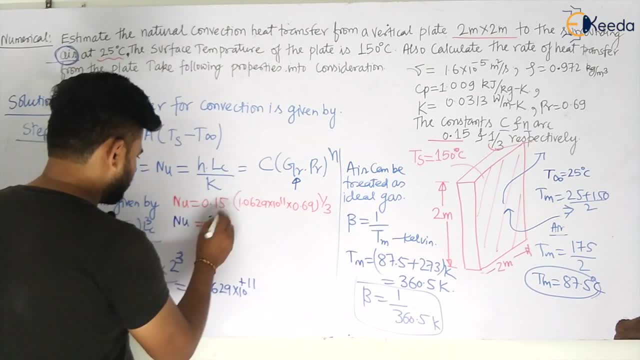 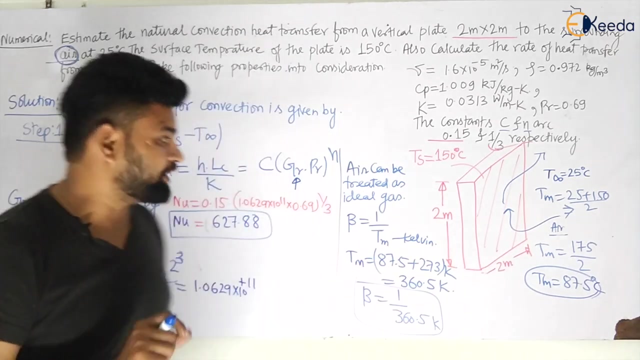 an assert number equal to that is 627.. Zero point 8, my dear students. So from this can I calculate the value of h? my dear students, Yes, I can calculate the value of heat transfer coefficient, that is, your h, and this will. 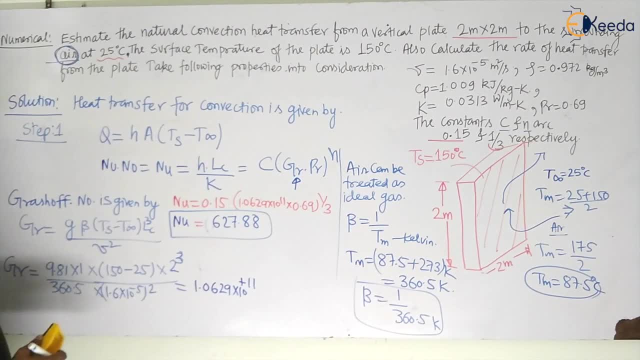 become equal to how much? Let us see. So let us calculate the value of heat transfer coefficient. So let us see the calculation for second step calculation for heat transfer, calculation for each task of coefficient h. So we know that h into lc by k fluid, k air, which is 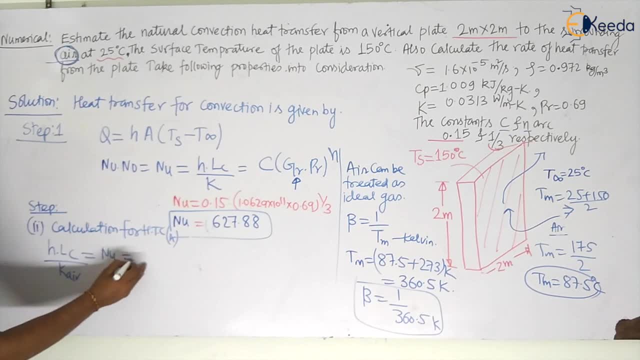 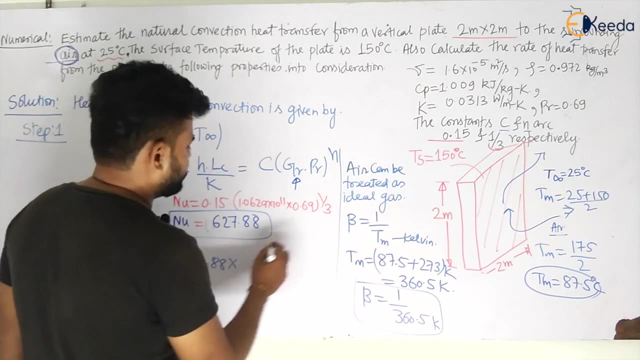 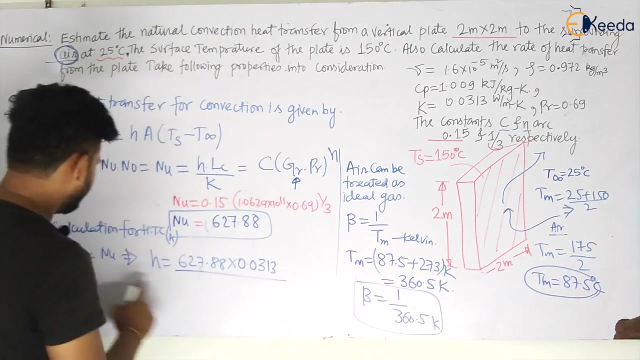 given is equal to nothing but Nusselt number, So this will be given by. h- is equal to 627.88, multiplied by k of air. conductivity of air is given to be how much? So this is given to be 0.0313, divided by the characteristic length, which is nothing but 2.. So, multiplied, 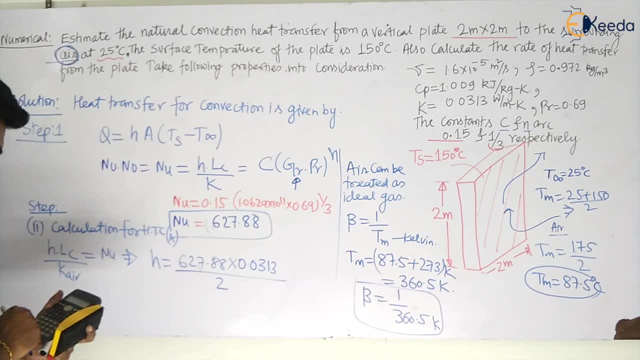 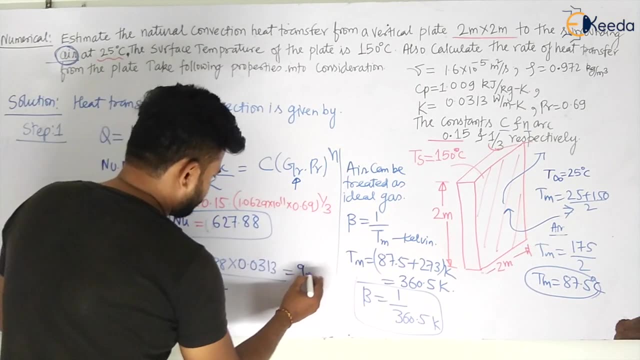 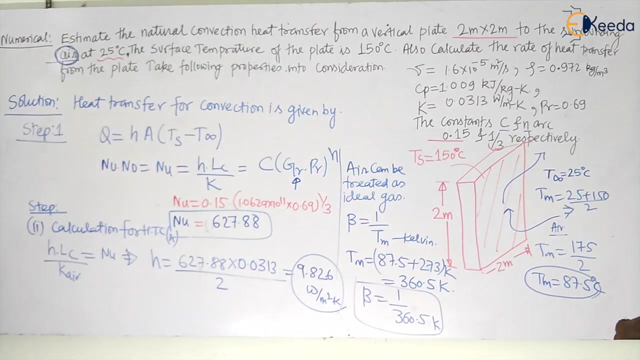 by 0.0313, divided by 2, and the value of h will come equal to 9.826 watt per meter square Kelvin. So now we know the value of h by the assurances. Now we know the value of h Can. 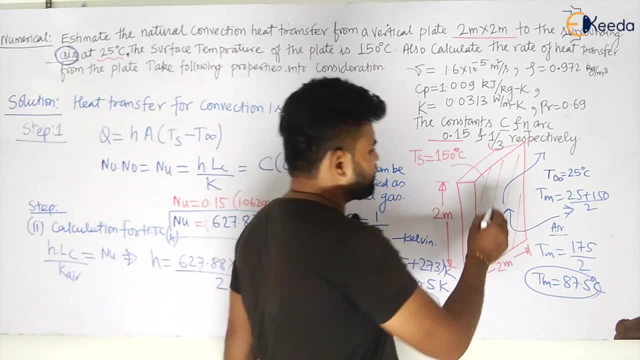 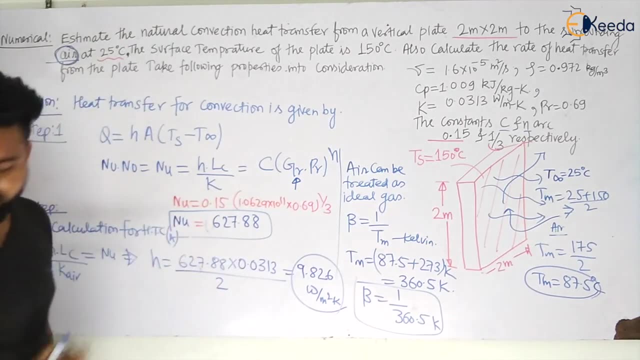 we calculate the heat transfer. Yes, So what will be the heat transfer from this side? So we can easily calculate, because we know the area, we know the temperature difference and we know now h. So let us calculate the heat transfer, my dear students. So the heat transfer, in this case, will be given by 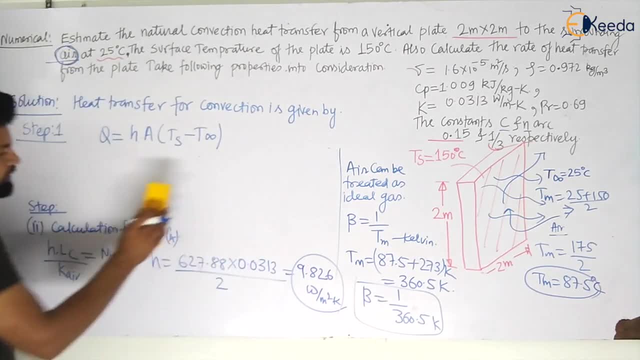 this. let us see. So the heat transfer, in this case, will be given by: q is equal to h, which is given to be 9.826, into area. What will be the area? 2 meter into 2 meter. in this direction, my dear students. So this is the area, So this is the area, So this, 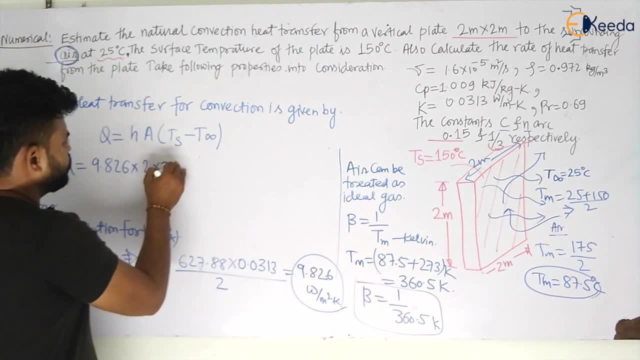 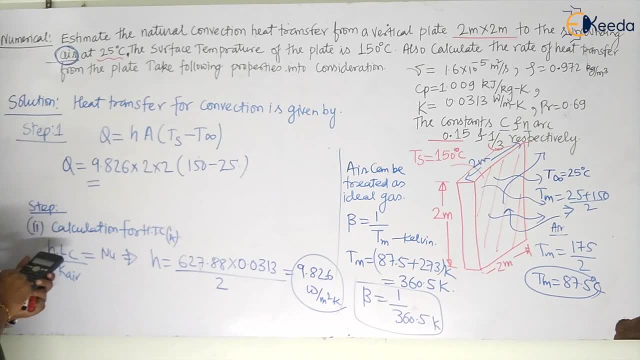 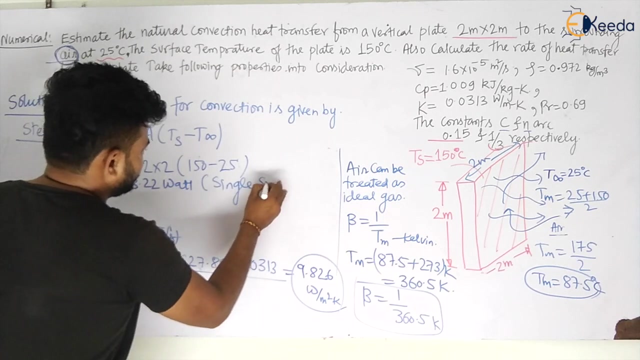 let us calculate the value So multiplied by 4 into 125.. So the value of heat transfer will be 04913.22 watt. and that is for single side. my dear students, that is for single side. So at two times you can do the mistake. at beta, delta is equal to 0.5 kilometers. 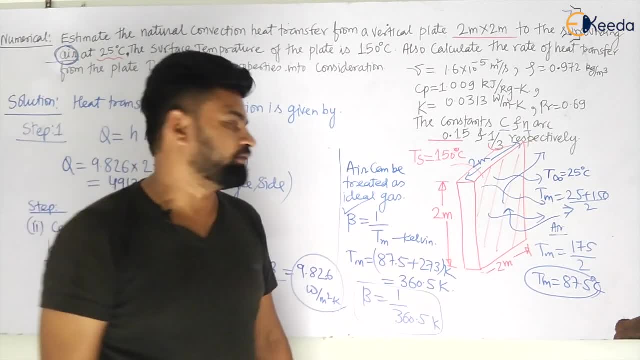 per second. So that can be calculated by plus, minus or minus. So this is the value of h. So let us calculate this value. So, as you can see, any value here is equal to, Because lap filter must be in Kelvin at second. the value is in for single side. this is: 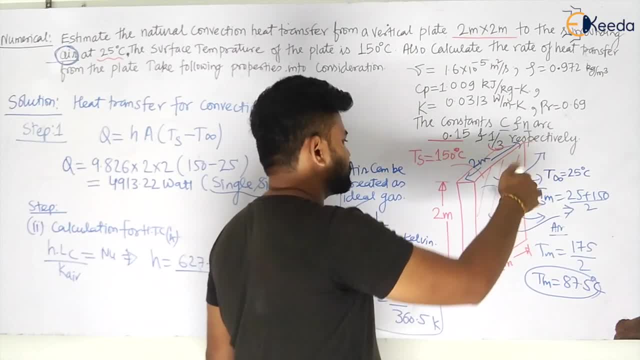 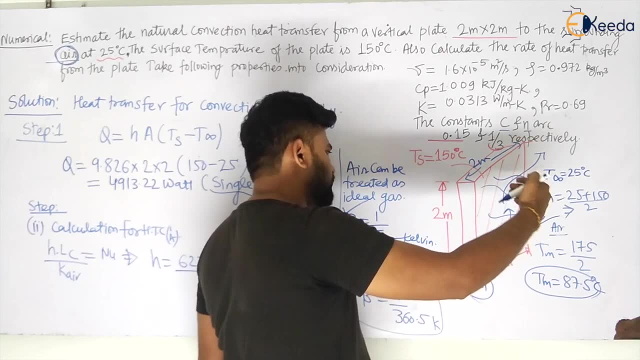 Now, what will be the total heat transfer? The heat transfer will be given from this side also, because this thickness is not given. So what will happen? So there will be heat transfer from one side, there will be heat transfer from other side of this plate. 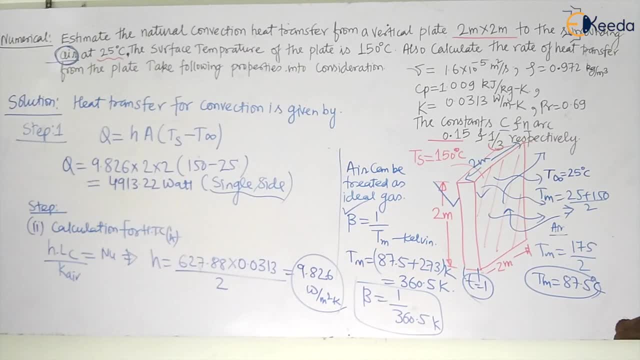 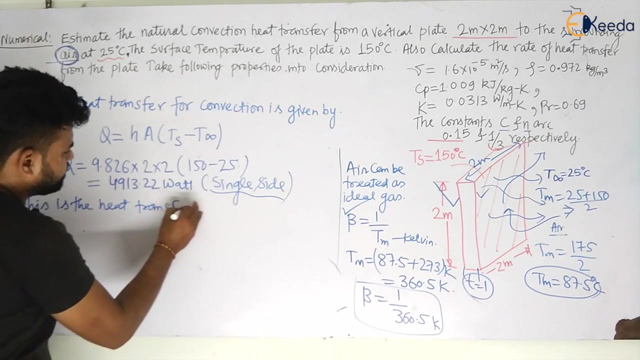 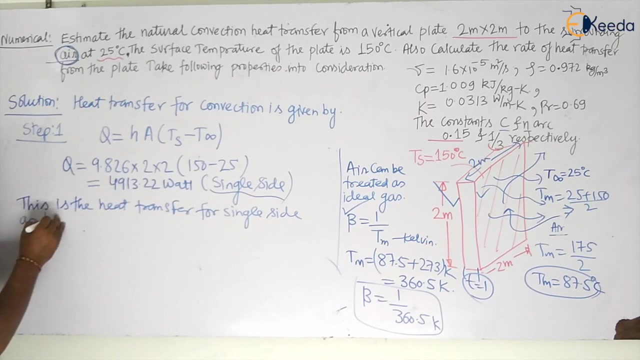 Other side of this plate. so total heat transfer will be given by, will be given by. let us see. So this is the heat transfer for single side, So as other side plate is having same properties, plate is having same area and same properties.